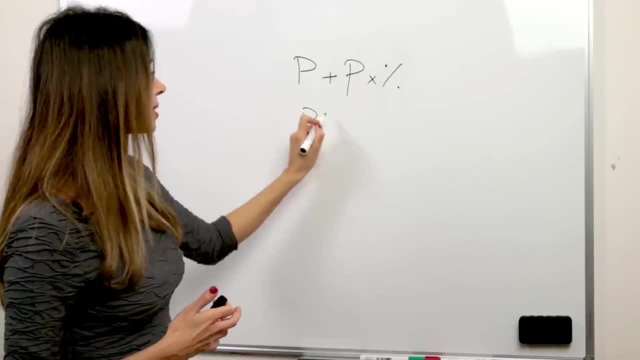 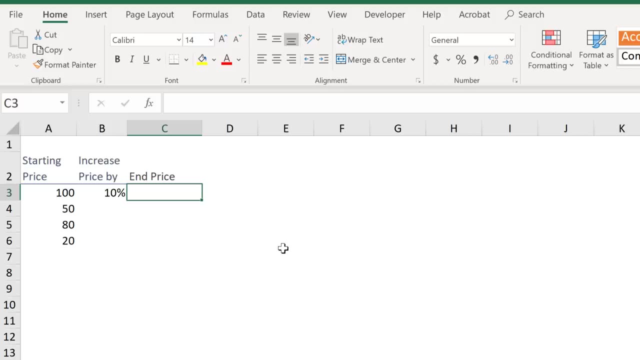 this is to factor out the price, So it's price times one plus the percentage, right? So that's another way of writing the formula. So in Excel this would be starting price multiplied by one plus percentage change. close bracket, press enter. So if my starting 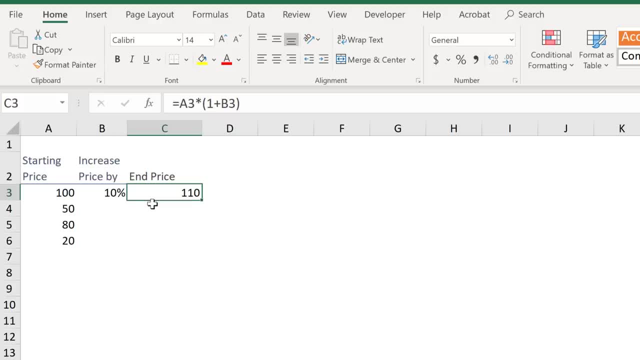 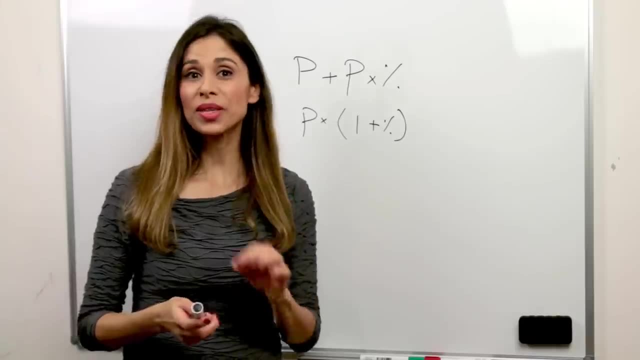 price was 100,. I increase price by 10%, I get 110.. If this was 5%, instead, I get 150.. In Excel, there's one thing you have to be aware of, and that's how you input your percentages. 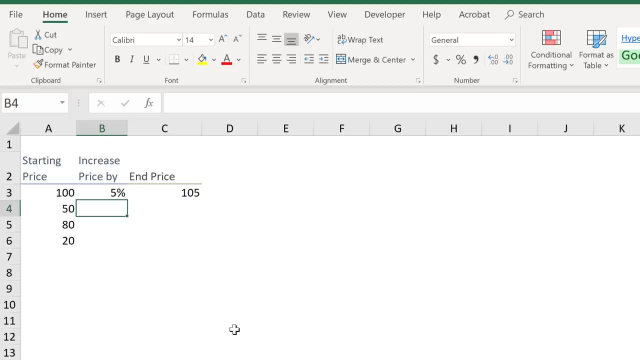 One method to input percentages is to add it while you type. So if I come here and type in 20,, followed by the percentage sign, and press enter, the cell is automatically formatted as a percentage. Another option is to input it as a decimal, So 0.05 translates. to 5%, right? So if I was going to pull this out, I'm going to add a decimal. So 0.05 translates to 5%, right? So if I was going to pull this out, I'm going to add a decimal. So if I was going 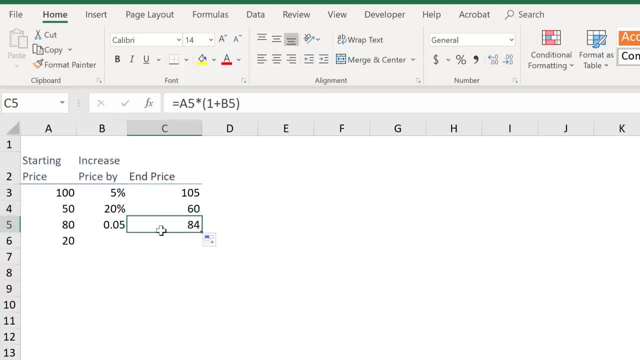 to hold this formula down. we can see it adds up correctly as 5%. Now I can change this to a percentage and I get 5%. Now another thing you can do is to format your cell as percentage first, before you input your full number. But don't do it. the. 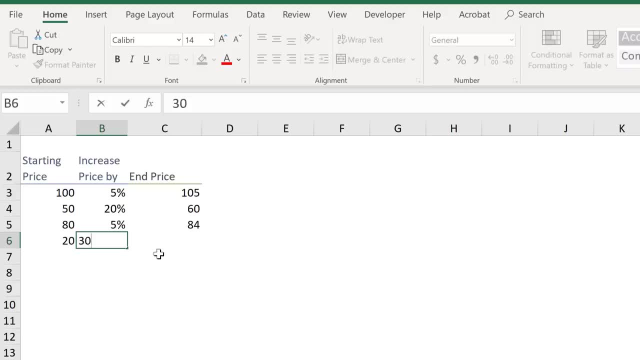 other way around. So for example here if I was going to input 30, then I decide this should be a percentage and I click to format this as a percentage. I get the wrong number Right. So if this was already formatted as a percentage, I go in and input 30, then it works fine. 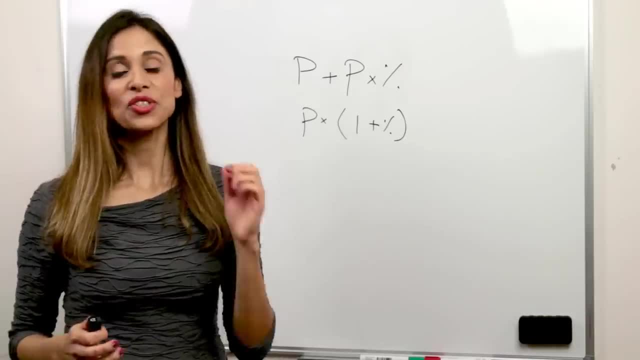 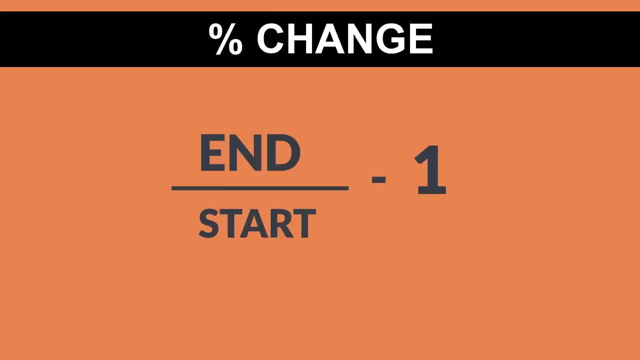 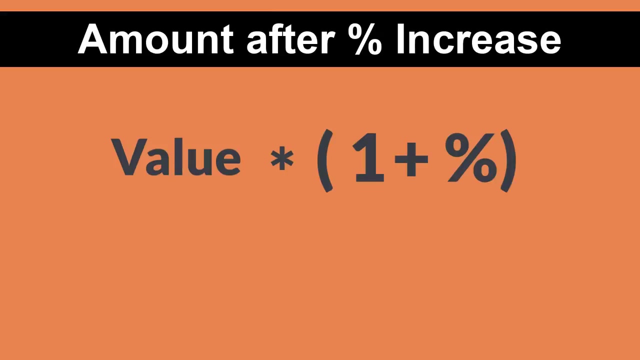 Okay, so let's just pull this one down too. So that's it. Just remember. for a percentage change, it's new divided by old minus 1, or end divided by star minus 1.. For a percentage increase, we have the formula: your value multiplied by 1 plus the percentage. 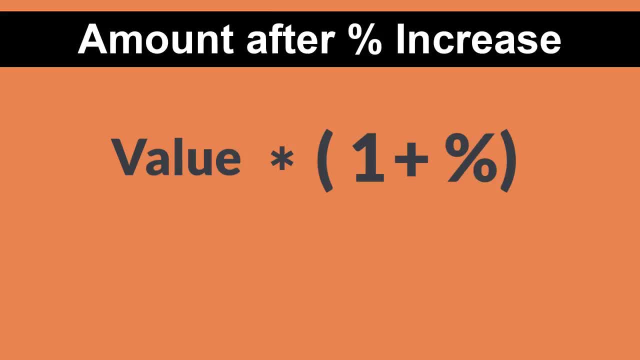 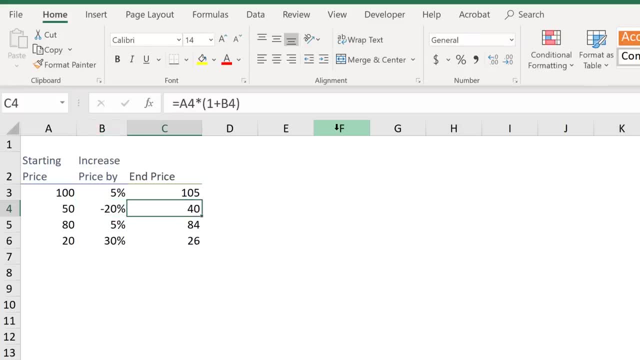 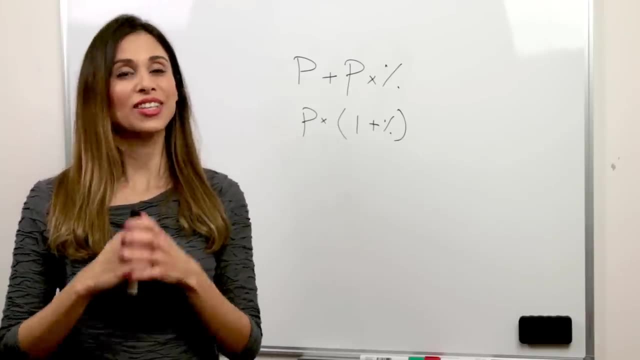 change And if it's a percentage decrease, it's your value times 1 minus The percentage change. But if you input your percentages negative in Excel, you can use the same formula, just drag it down. So the next time you're asked to calculate the monthly or yearly change, you know how.